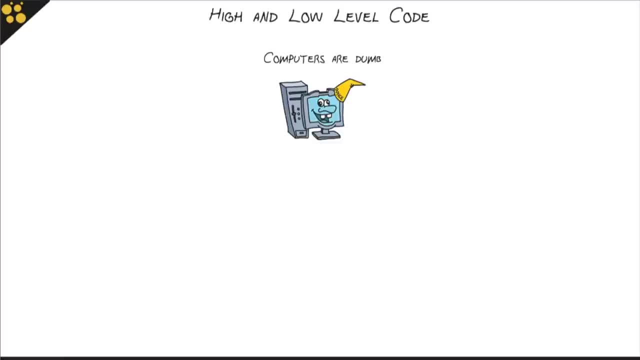 clear and explicit as possible, so that the computer does exactly what we intend for it to do. So to that end, machine language, the language that actually instructs the computer on what to do, is pretty esoteric. It looks something like this. I've got on screen here: 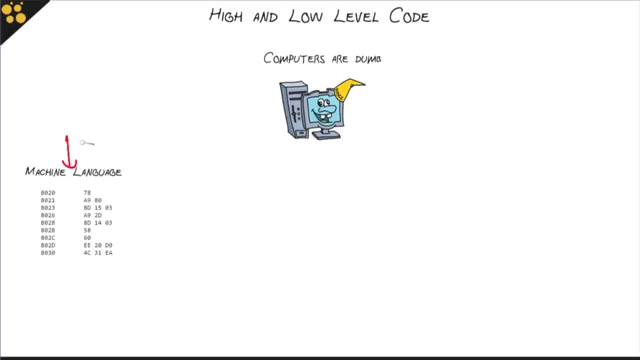 And if you're looking at it, saying, well, that's not a language, that's just a bunch of numbers. yeah, you're right, This is binary language, This is machine language and it is a set of instructions for a particular computer. 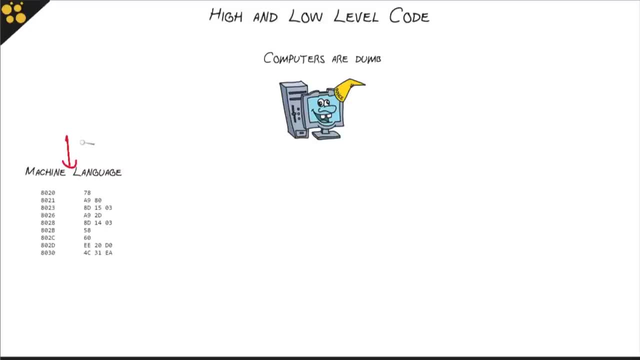 I don't have the slightest idea what it does, What these instructions are telling it to do. The point is that no one really does. No one really programs in machine language, because it has to be so hyper-precise and so specific that it's not especially useful. 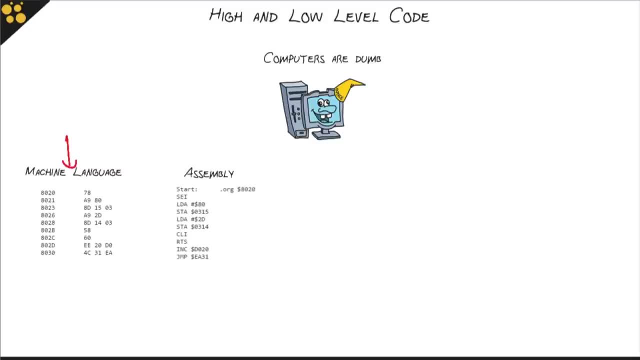 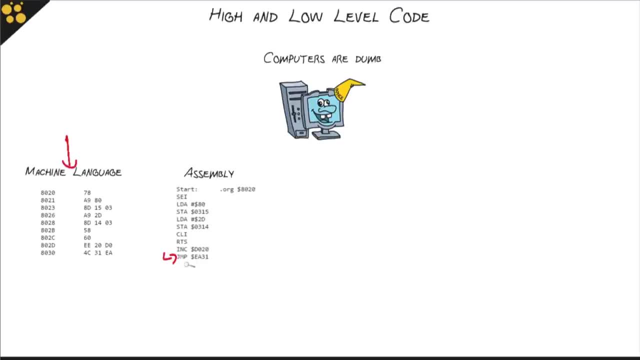 We're going to look at a couple of other things. We're going to look at a couple of other things. Assembly is one step up for machine language And before assembly can be interpreted by a computer- yeah, it still has to get turned into machine language. 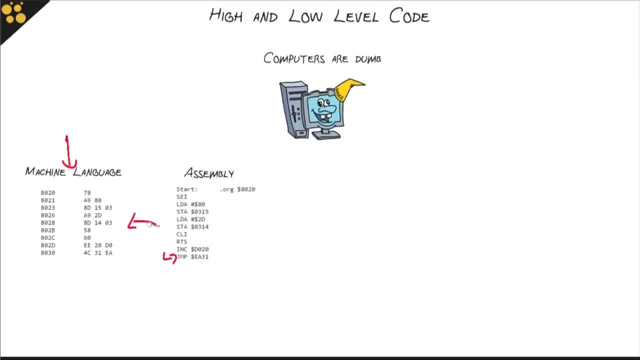 But when the need arises to write really detailed, very specific instructions to a computer assembly, is the language that is used that is chosen. There is some marketplace out there for assembly programmers. If it's the kind of thing that interests you, I expect that you would want to find out more. 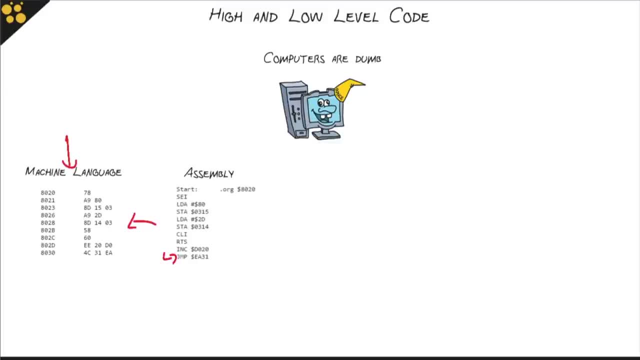 about it and really find out if it's something that you want to do. But it's not a huge marketplace of coders. Most coders, most programmers, are working in a higher-level language, the languages that we just mentioned, that you've heard about: Python, PHP, Perl, Java. 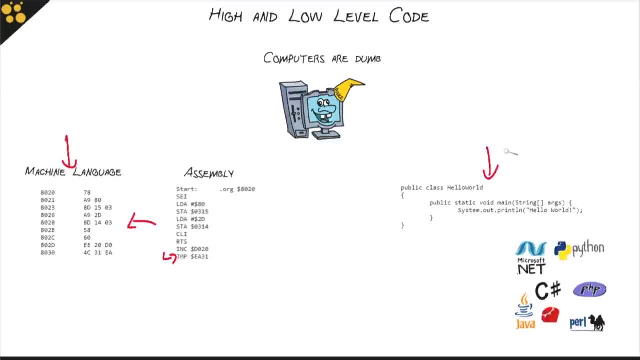 These high-level languages look something like this: Now, they're still not English, They're not a natural language, But they are closer to a natural language. They kind of bridge the gap between the language that you and I speak, which is incredibly arbitrary, incredibly ambiguous and not very easy for a computer to understand, and the 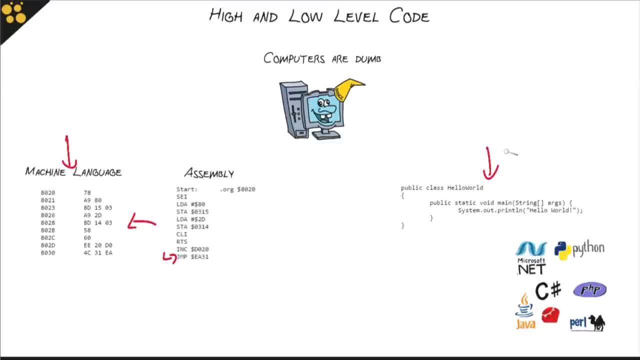 machine language. It is totally impossible for us to understand So in a high-level language like you see here. this is an example of C++. I believe you see some English words in here: class public static system. You may not understand what this is doing, but you would recognize those words as English. 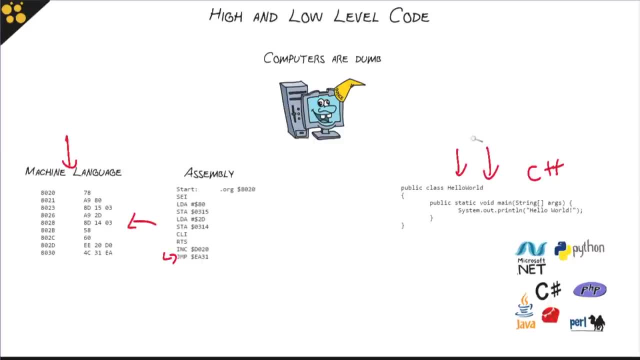 words. Consequently, this code right here is a lot easier to understand than any of this code over here. It boils down to a level of what we like to call abstraction. The direct computer instructions are less abstract, While the high-level languages are more abstract. 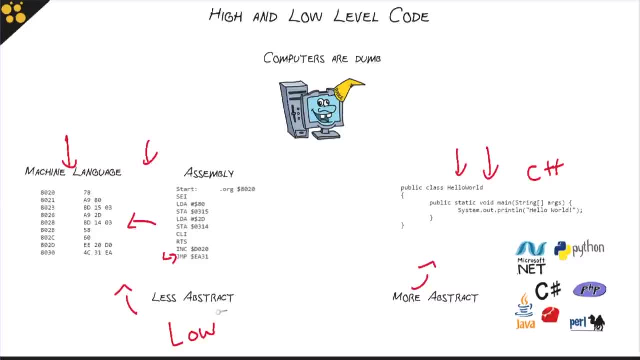 And that's really what the breakdown is here. These are the low-level languages down there: assembly and machine language And everything else over here is a high-level language. The high-level language allows us to use some familiar words and some familiar structures of grammar, at least if you're familiar with the English language. 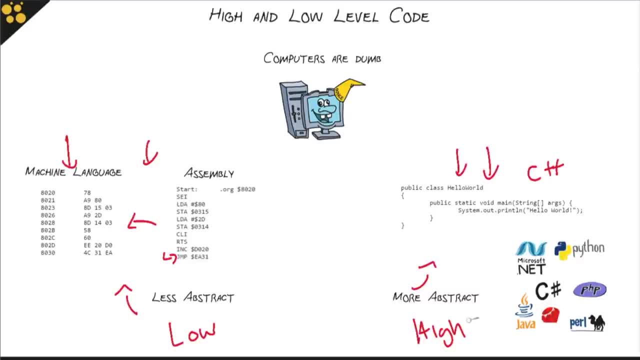 And by using those it's easier for us to write, but we still have a lot of structure forced upon us so that our instructions to the computer are very explicit and can be turned back into a low-level language. So that's the breakdown here. 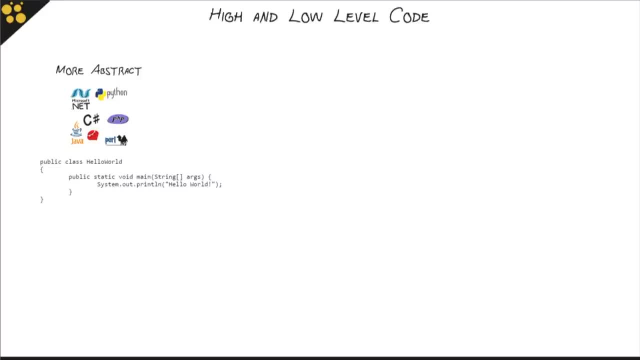 A low-level language, And that last phrase right there turned back into is really critical for understanding how programming languages work as well. After all, a more abstract language like C++ that I've got on screen here is useful, but it can't be understood by the computer. 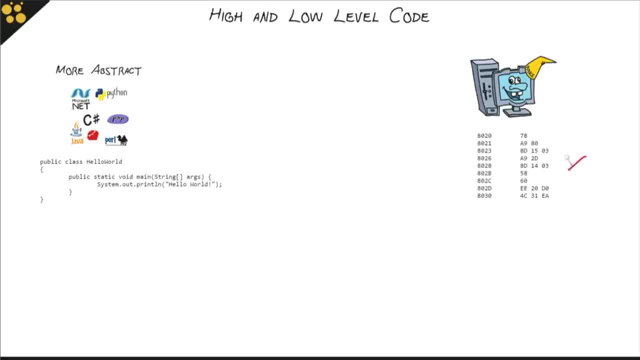 The computer still ultimately needs machine language. This is the instructions that the computer needs. So we've got to turn this into that somehow, And I've mentioned this before in another video. but yeah, this is done with something called a compiler. A compiler is a piece of software. 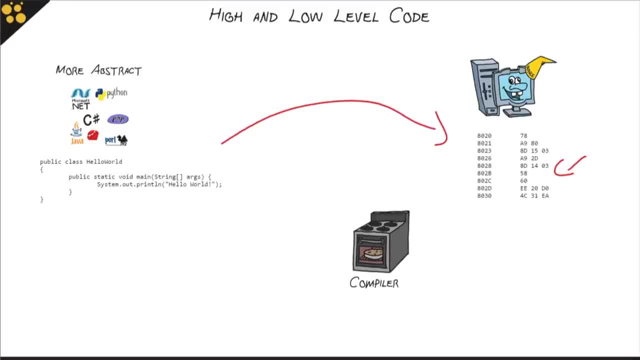 A compiler is a piece of software that runs on your computer After you've typed up all of your source code. it takes that source code and it turns it into machine language so that the machine can actually execute the code that you've written. It can perform the instructions that you've provided inside of that source code. 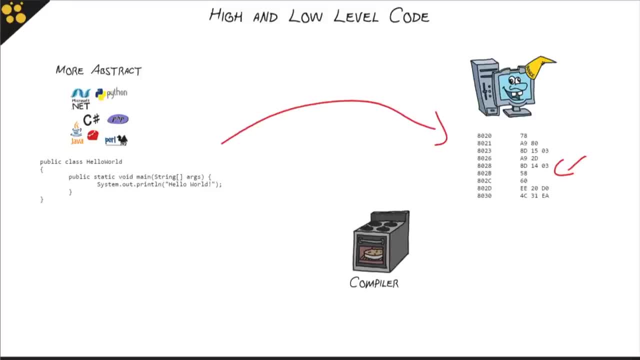 The analogy I like to use- and you see, I've got the oven here- is sort of like baking. Source code is like your individual ingredients, your sugar, your flour, your eggs. You can't eat raw eggs, right? I mean, I guess you can, but it's gross. 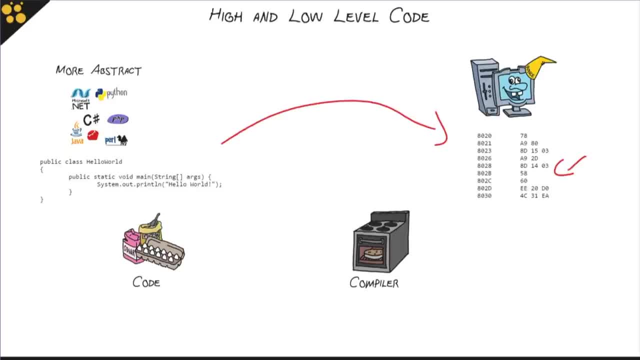 No one's doing that, And the computer can't eat the raw eggs either. First they have to be well mixed, Yeah, Mixed together in something we call a linker- We're not going to talk much about that. And then, after they have been linked, they go to the compiler, and the compiler bakes. 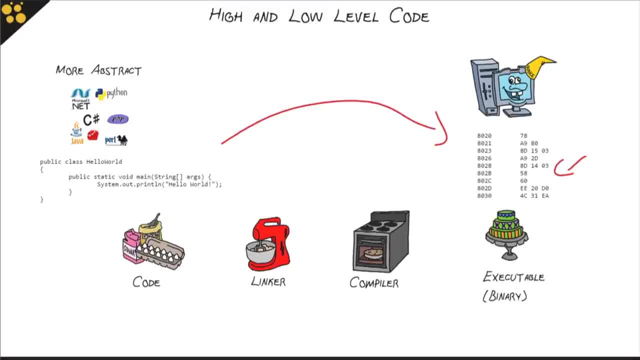 them And once they have finished being baked, now it is an edible cake. It is something that the computer can consume. We call this an executable or a binary, And this is the file that is written out in these machine languages, very esoteric, specific. 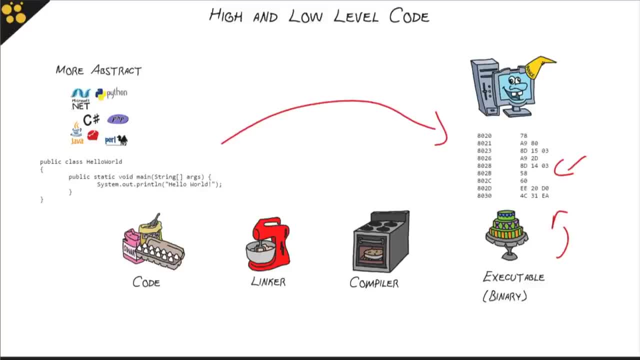 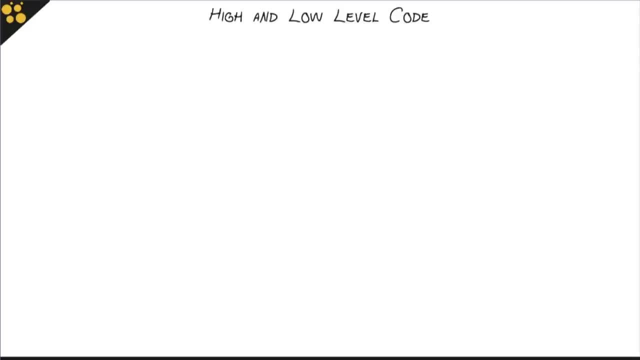 but difficult to parse language And all high level programming languages have to go through this process before they can be executed. But all high level programming languages are not the same. Just to break things down a little bit further here: when we get to an executable, to a binary, 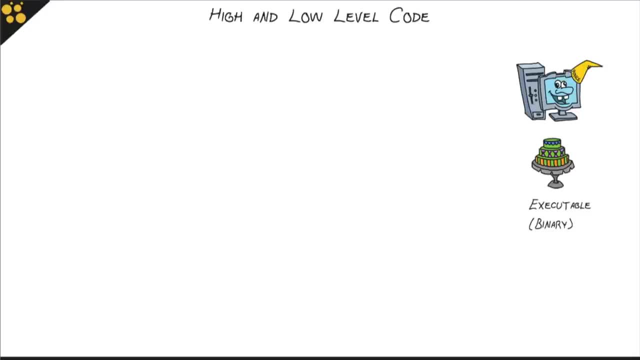 that's always the end goal of any program that we write. It has to be turned into an executable before the computer can consume it. It has to be machine language. There are really kind of three different types of languages in general that you're going. 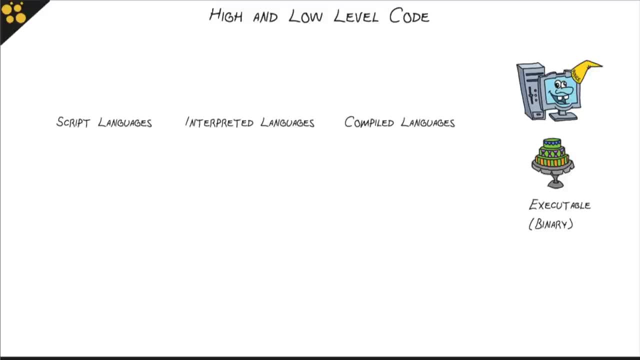 to work with at a high level, And that is scripting languages, interpreted languages and compiled languages. Now, what we have been doing is we've been working with a bunch of different types of languages, And what we have been talking about are compiled languages. 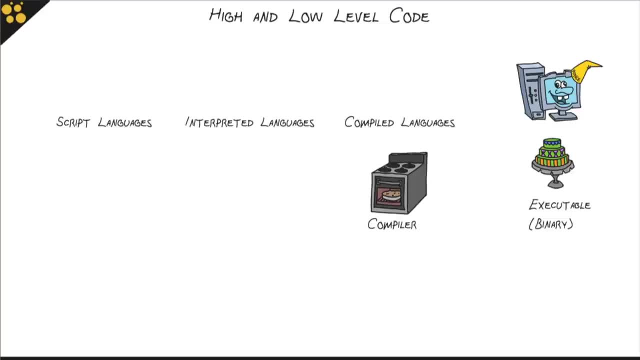 You write the code, You run them all the way through the compiler. It outputs a binary file, a literal file on the file system. that then gets delivered to the computer where it is going to run. But there are earlier iterations that you can engage with as well. 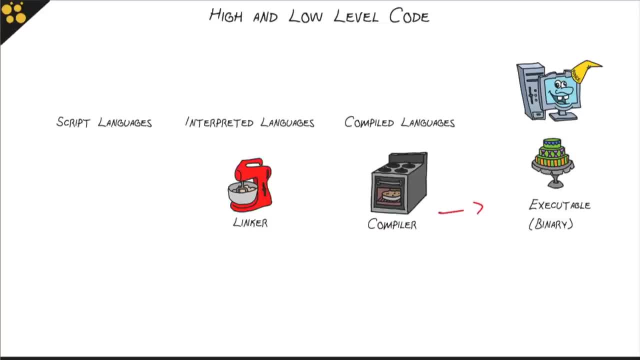 Interpreted languages, for example, stop after the linker An interpreted language, and the primary ones of these are Java and C sharp don't get compiled. They get turned into this sort of semi-parbaked, half-compiled file, often referred to as bytecode. 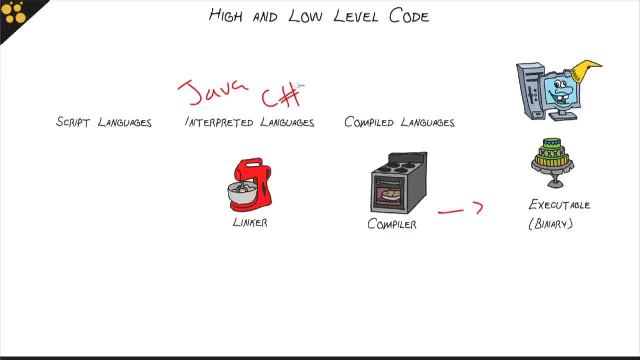 And it's that which is delivered to the end computer where it's going to be run. Now you may be thinking to yourself: well, bytecode is not a binary. A computer can't eat that half-cooked cake, And you're absolutely correct. 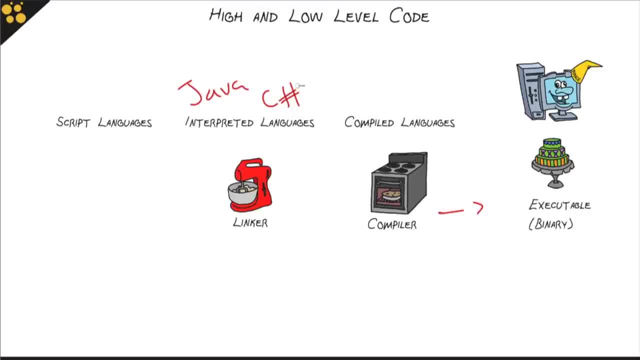 The final step- compiling- actually happens on the target computer. It happens on the computer that is executing the code And it happens while it's executing it. We call it just-in-time compilation. That's really important, because what that allows us to do is write one program and compile.